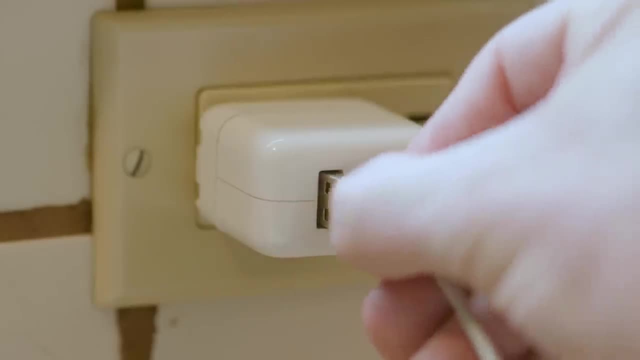 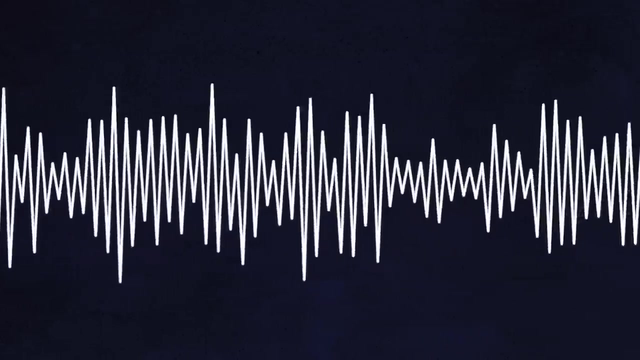 like the 50 or 60 hertz signals that come from our wall outlets, or even audio signals that go up to 20 kilohertz, which is the maximum frequency humans can hear. the associated wavelengths are very long If a signal travels at the speed of light through a cable. 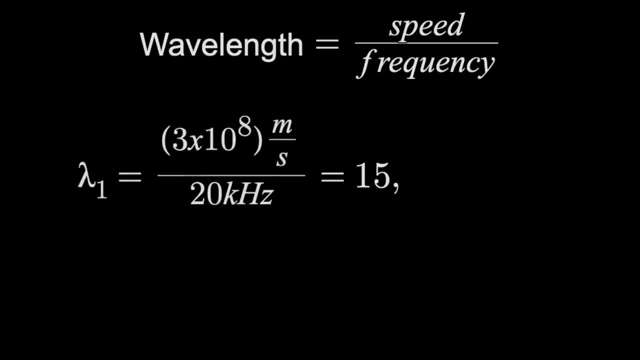 even at 20 kilohertz the wavelength comes out to 15,000 meters And that is most likely much longer than the cable it is going through. But bump that frequency up to 100 million hertz, the frequency of radio waves. 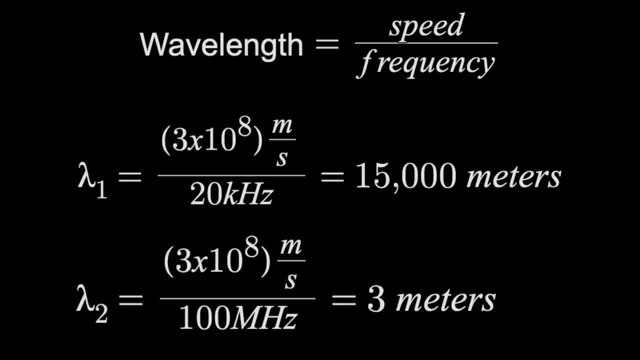 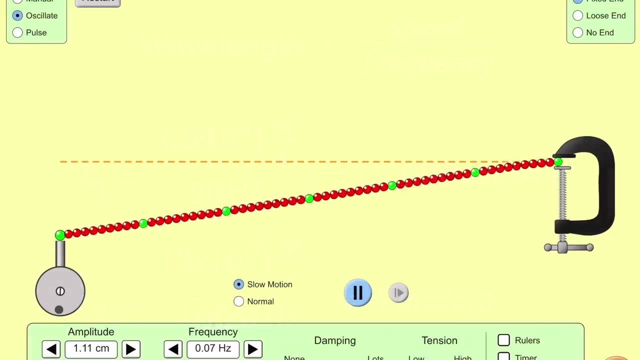 and you get three meters- And this is much more comparable, maybe even shorter than the cable it will be traveling through- And when that happens, you're gonna get reflections within the cable, Just like if I take a rope and pulse it very slowly. 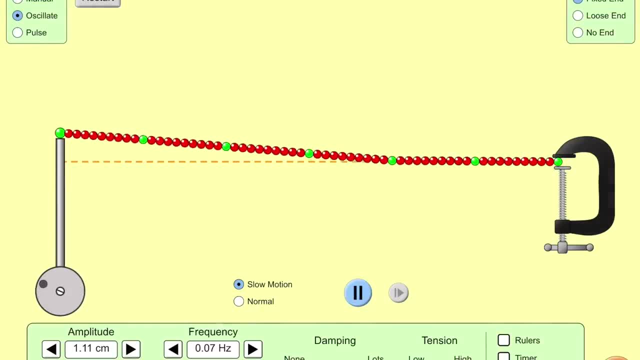 the rope moves in a very predictable way Because the actual wavelength is so much longer than the rope itself. But pulse that rope faster where the wavelength is comparable or shorter than the rope, and then you're gonna get reflections and things get more complicated. 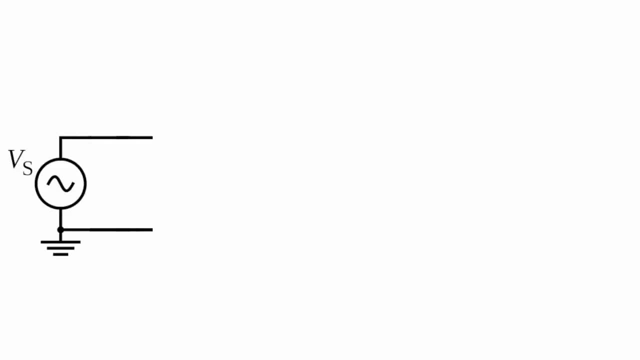 So in the circuit world you might have some high frequency input, Maybe for radio, television, satellite communications and so on, Which goes through something called a transmission line, Just a specialized cable often used for these high frequency signals Until that signal gets to some load. 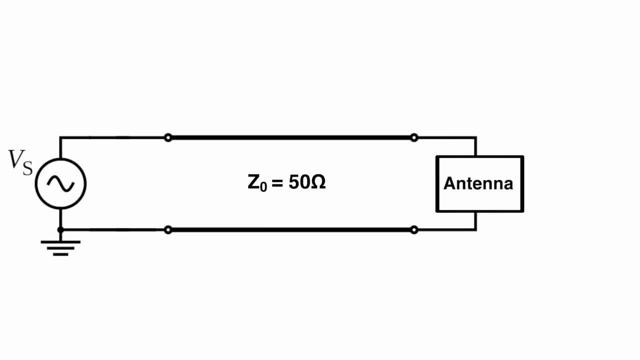 Maybe an antenna to be transmitted Now that transmission line is going to have some associated impedance to it. 50 ohms is often what is used, So really just a resistance, And this is a fundamental property of the cable, Determined by material properties and physical dimensions. 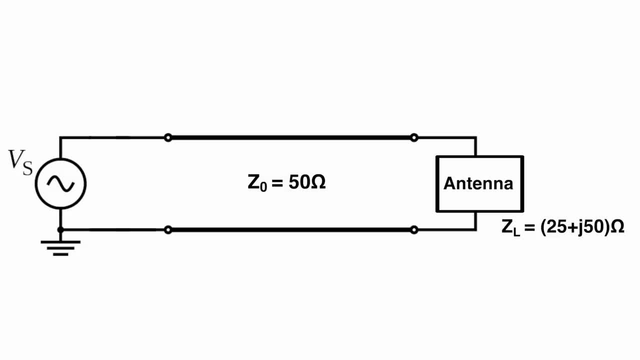 And then the antenna is also gonna have an associated impedance, Likely both a real and imaginary component, Meaning it has some resistance and some capacitance or inductance. Capacitance and inductance are represented with an imaginary number And EE's use J instead of I. 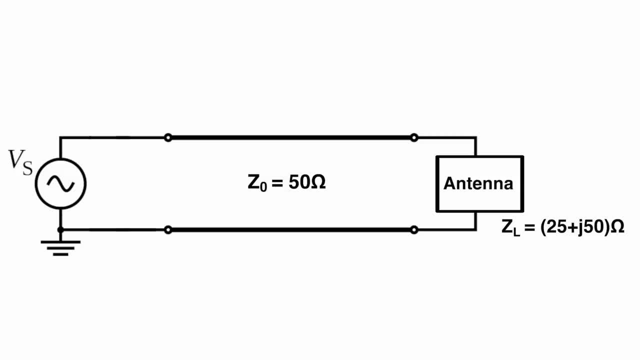 cause I is used for current Okay, so what we have here is kind of like a rope attached to a bigger rope, Both free to quote, move or change voltage and current, But they have different properties. So what would happen if we pulsed that? 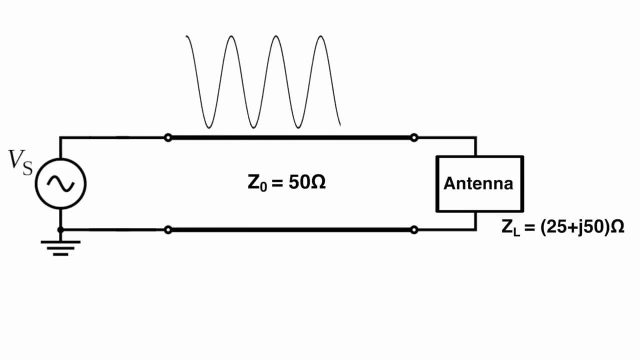 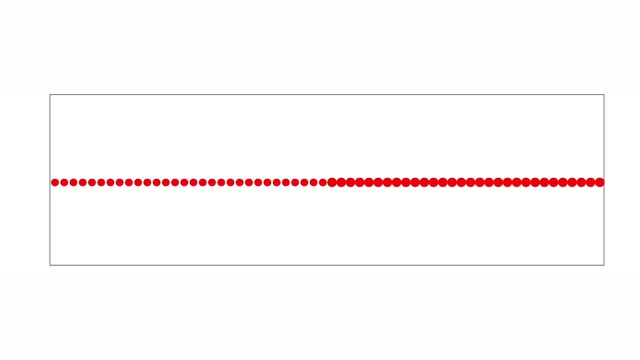 We'd send a wave down the first rope and it goes until it would hit that junction. Then at that point, some of the wave's energy will be reflected back, while some will transmit through to the antenna. You can see that visually here. 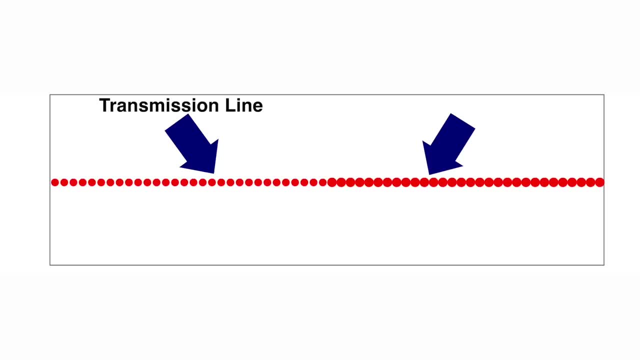 We got smaller rope attached to bigger rope, Transmission line attached to antenna. Send a wave down. Once it hits the junction in the middle, boom. some energy goes through, while some is reflected back. We typically don't like those reflections. We want as much of the signal's power as possible. 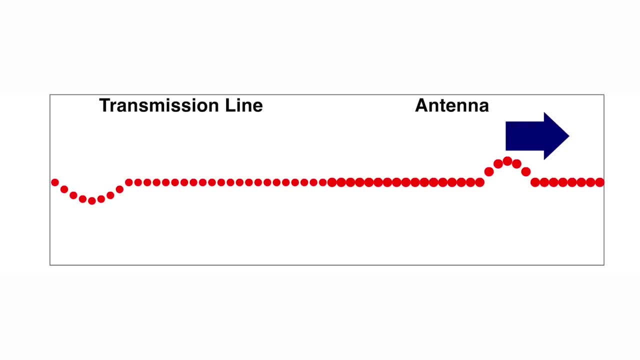 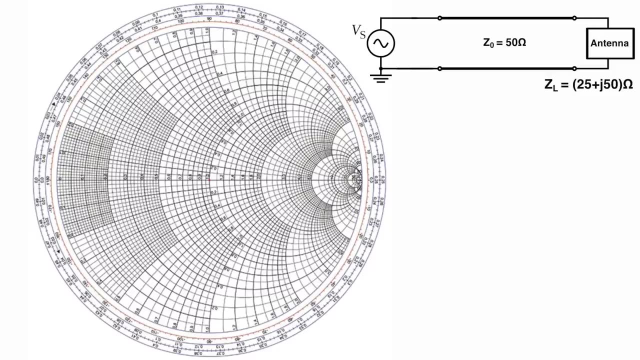 to get to the antenna so it can be transmitted, And that's where the Smith chart comes in. This tells us the parameters we need to know, Like how much voltage gets reflected versus how much is transmitted. So here's a quick example with the numbers shown here. 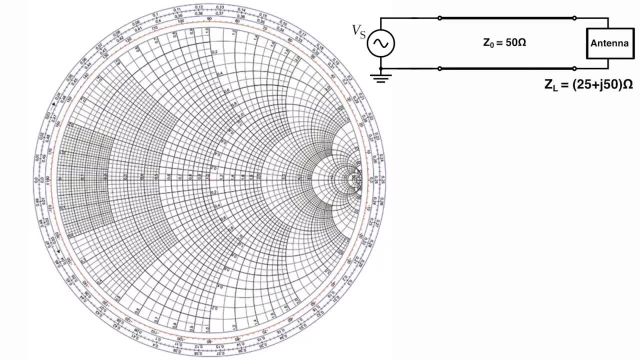 The first thing to note is, as chaotic as this looks, you're really just looking at a bunch of circles. You got these ones that are fully inside the Smith chart that have to do with resistance, which we'll see in a sec. Then these curves are also just circles. 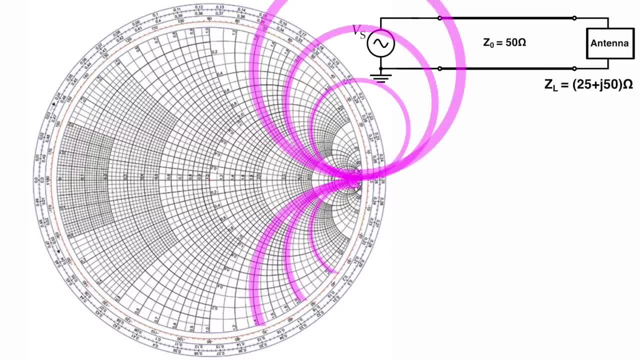 Well, the portion of them inside the Smith chart, And they have to do with reactance, The capacitive or inductive part of the load represented by an imaginary value. Anyway, step one with the Smith chart is to take your load impedance and divide it by the transmission line impedance. 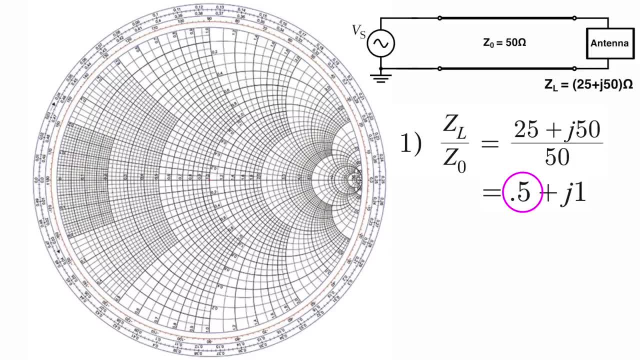 Then you take the real part of that and find that value on the horizontal axis Hard to read. but 0.5 is right here, which is on this circle which we're gonna highlight Again. these circles are all of constant normalized resistance. 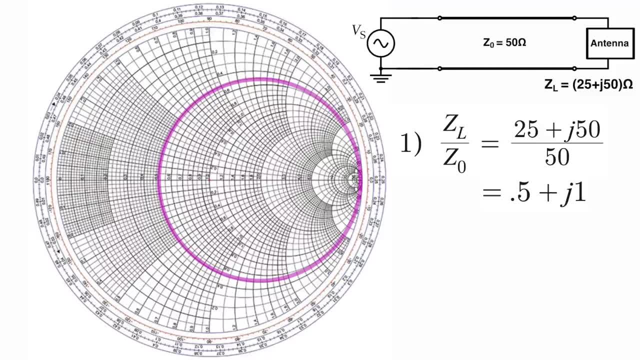 that all correspond to the real component. Then for the imaginary part you find that value out here along the perimeter of the Smith chart, In our case positive. one can be found right here. The top is all positive values, aka inductive. 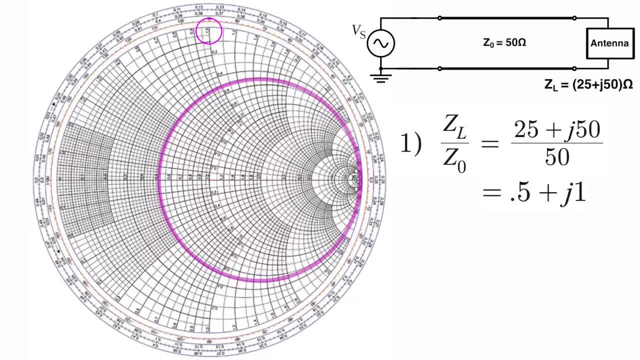 If the value was negative one, then we find that on the bottom half of the Smith chart We'll then highlight that associated circle of constant reactance. Again, those are always for the imaginary component. Then the intersection point of those two circles is gonna tell us how much of our wave. 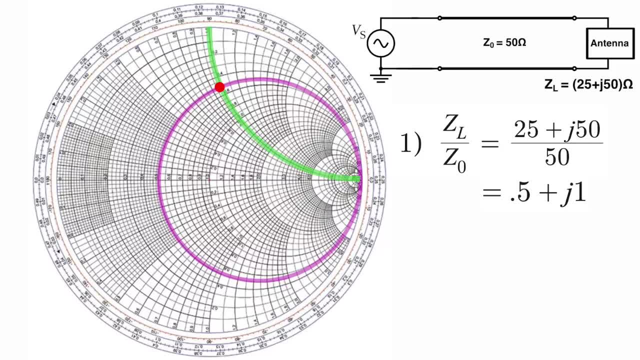 will reflect back from the antenna And that's found by looking at the distance. that point is from the center of the Smith chart, taking the very outer circle to be the unit circle distance of one away. So in this case- and you'll typically have a little scale- 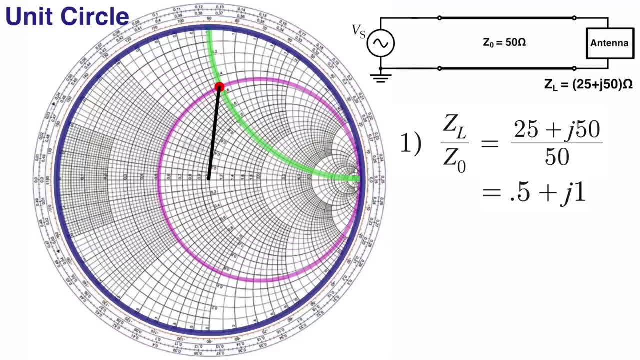 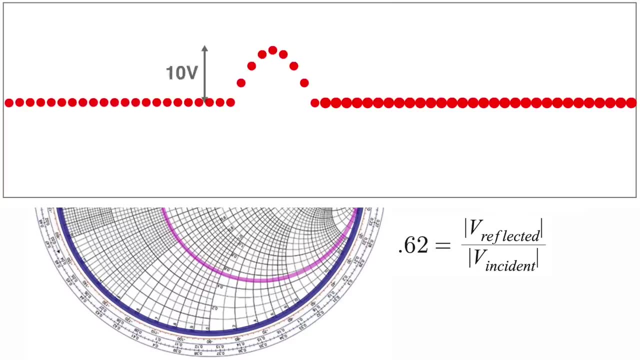 below your Smith chart. that distance away is just about 0.62, meaning the ratio of the reflected wave voltage to the incoming or incident wave voltage is 0.62.. So if the incoming wave had an amplitude of 10, the reflected wave will have an amplitude of 6.2. 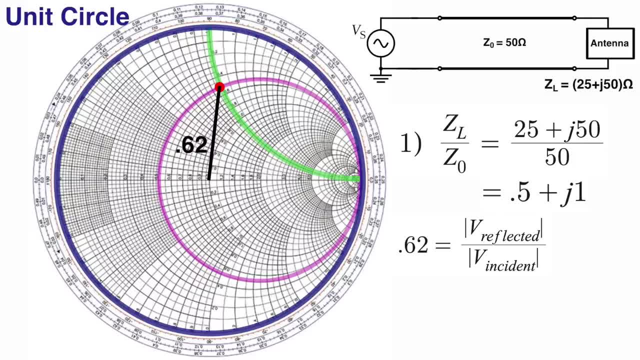 So the smaller that ratio is, or the closer this intersection is to the center, the better. That means less of the wave will get reflected and more will go to the antenna. So if now the antenna's impedance was something like 45 plus J10 instead, 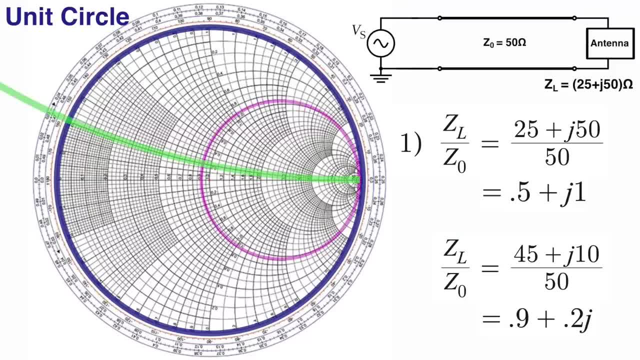 then normalizing that and finding the associated circles, we'd find an intersection point much closer to the origin, meaning less reflection. And that's because the impedance of our load is now more closely matched to our 50 ohm transmission line, The real parts being 45 versus 50 respectively. 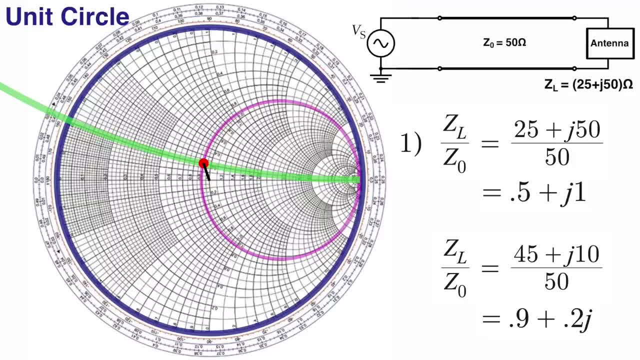 pretty close, And then the imaginary values are 10 versus zero, also closer than before. Now, if the antenna also had an impedance of just 50 ohms, they matched. then the intersection would be found at the very center of the Smith chart. 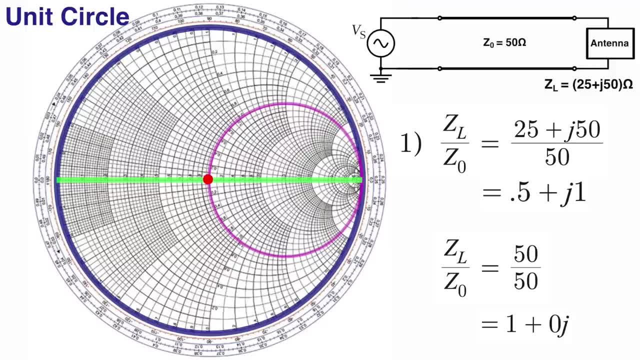 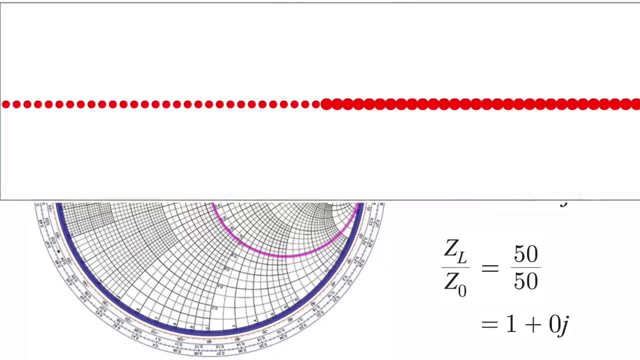 a distance of zero away from the center, meaning there would be no reflected wave, which is not a wave- exactly what we want. this would be like, instead of before, where we had different size ropes, we just had a rope tied to an identical rope. now there will be no reflection because, well, it's all. 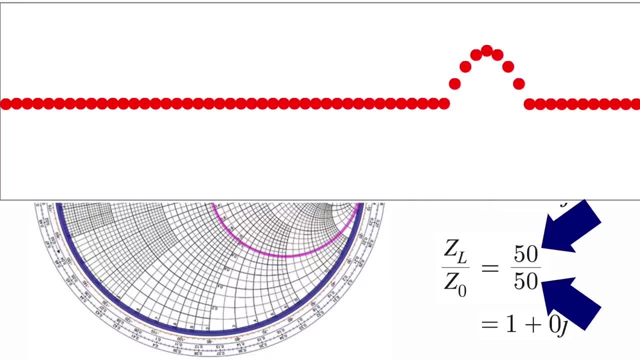 the same rope, so we'd like matched impedances or same size ropes, because all the energy gets through to our load, and this is actually the real use of the smith chart. when we have mismatched impedances that cause reflections, we can add things to the circuit that make the impedances.